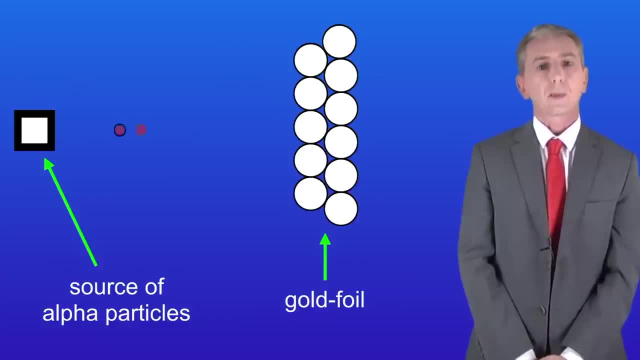 The first thing they saw was that most of the alpha particles passed straight through the gold foil without changing direction. Sometimes an alpha particle was deflected, In other words, it changed direction as it passed through the gold foil, like this, And sometimes an alpha particle simply bounced straight back off the gold foil. 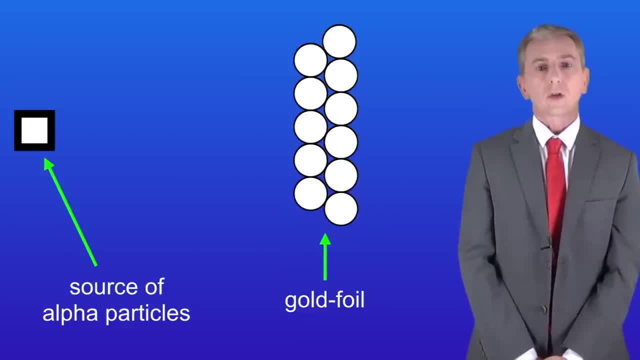 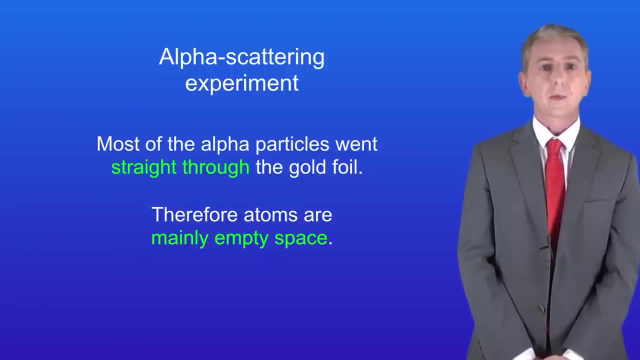 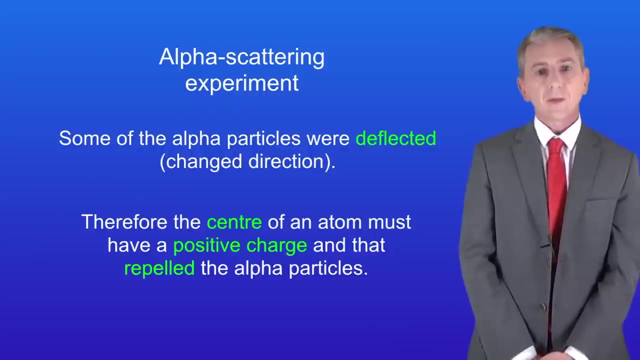 So let's look at what scientists worked out from these results. The fact that most of the alpha particles went straight through the gold foil told the scientists that atoms are mainly empty space. This meant that the plum pudding model had to be wrong. Secondly, because some of the alpha particles were deflected. this told the scientists that the centre of the atom must have a positive charge, and that repelled the alpha particles. 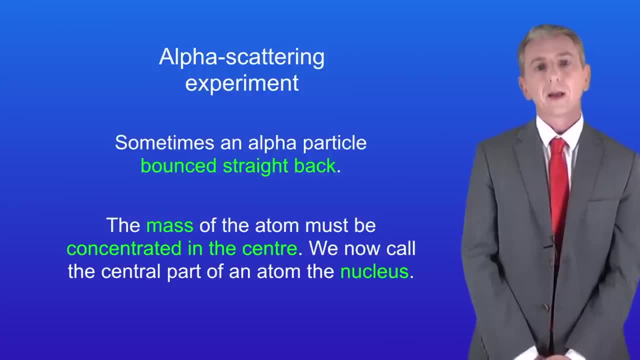 And finally because some alpha particles bounced straight back. this told the scientists that the mass of the atom must be concentrated in the centre. We now call the central part of an atom the nucleus. When an alpha particle collides directly with the nucleus, it simply bounces back in the original direction. 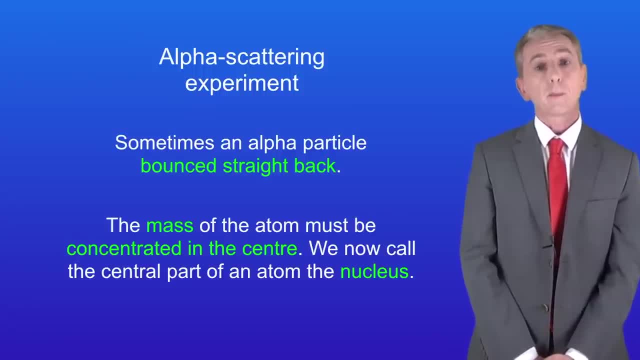 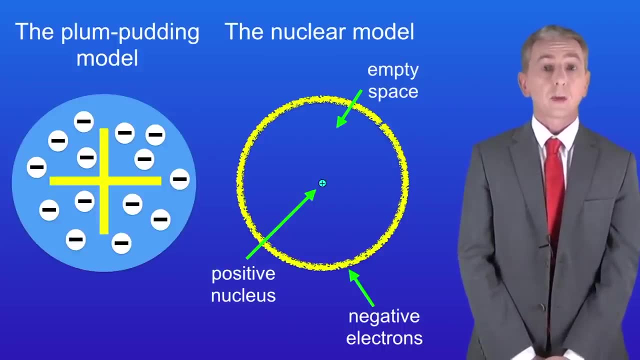 So from these results, scientists replaced the plum pudding model with the nuclear model, and I'm showing you that here. So most of the atoms simply empty space. In the centre we've got a tiny positive nucleus containing almost all of the mass, And around the edge we've got negative electrons. 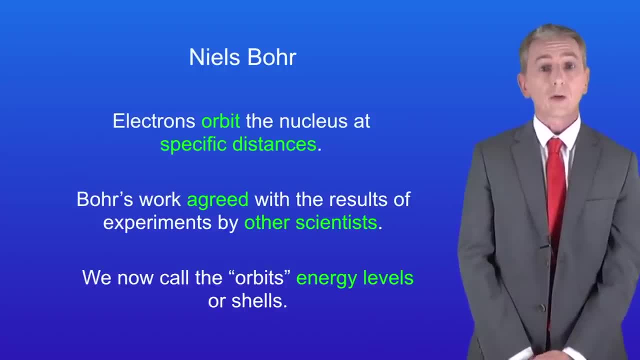 Now the scientist Niels Bohr proposed that electrons orbit the nucleus at specific distances rather than just in a general area. Bohr's proposal was accepted because it agreed with the results of experiments by other scientists. We now call these orbits energy levels or shells. 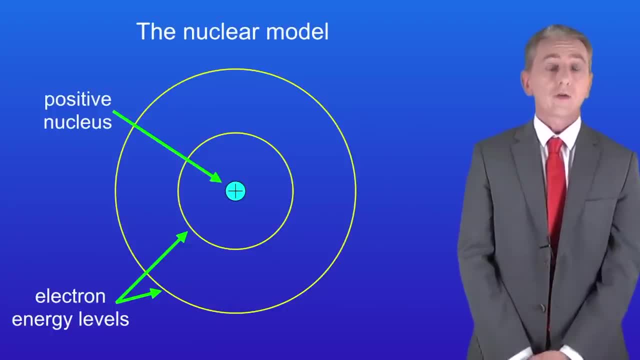 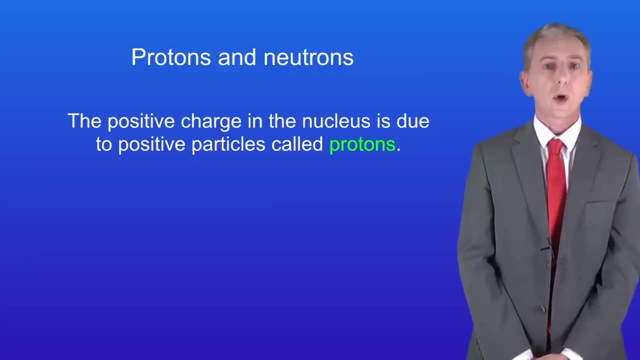 So here's the updated nuclear model with the electrons in energy levels. Several years later, scientists found that the positive charge in the nucleus is due to positive particles, which they called protons, And around 20 years after the nuclear model was first proposed, the scientist James Chadwick discovered that the nucleus also contains neutrons. 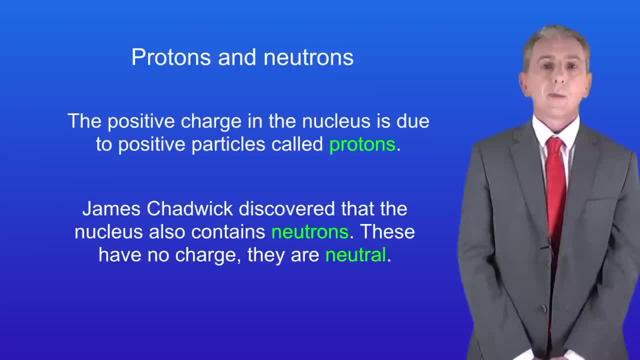 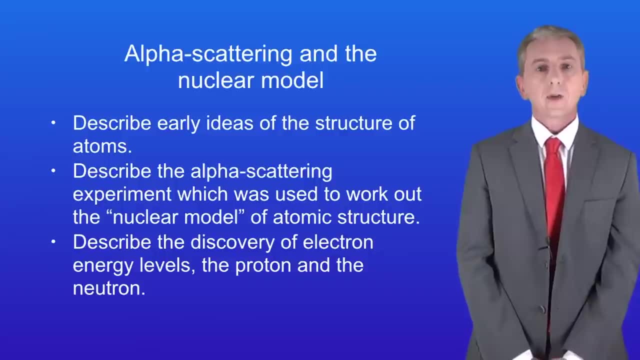 And neutrons have got no charge. they're neutral. Remember, you'll find plenty of questions on this topic in my vision workbook And you can get that by clicking on the link above. Okay, so hopefully now you should be able to describe early ideas of the structure of atoms.